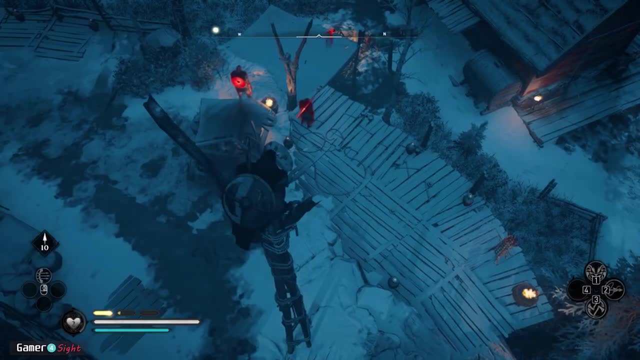 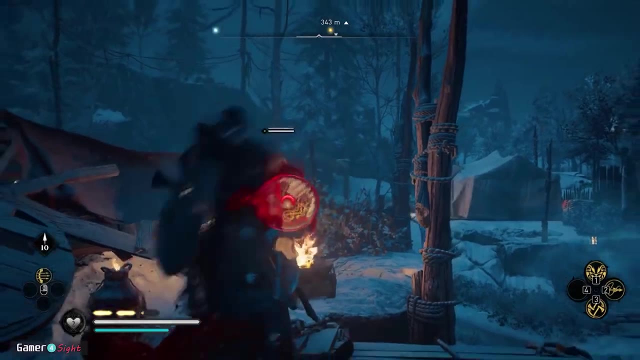 typically, we get bored. However, in games, a player doesn't only become bored if they have learned all the available patterns, but also when the patterns of the games don't match the player's personal interests, when the patterns are so simple that they seem trivial when they're so. 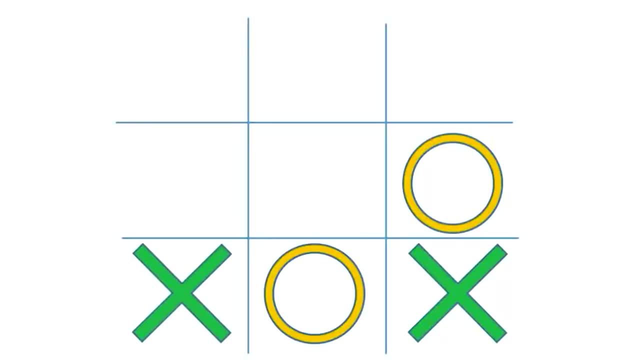 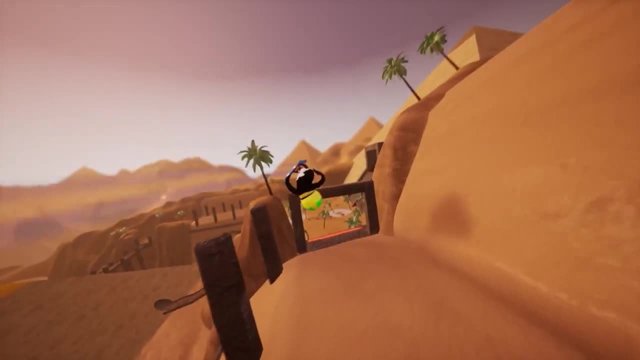 difficult, that they can't even be identified when they're revealed too slowly or too quickly, or when the player finds a way to cheat. They always find a way to cheat. So up until now, we've established that games are fun when they teach players to learn patterns which match their 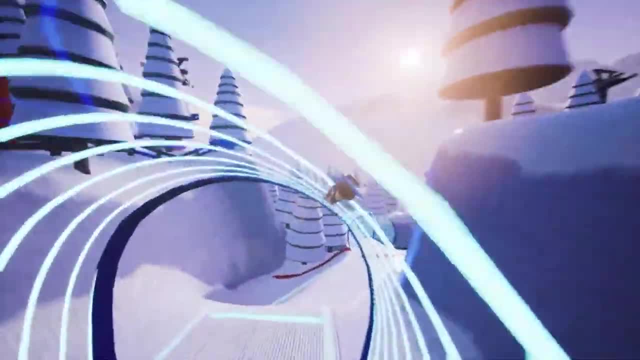 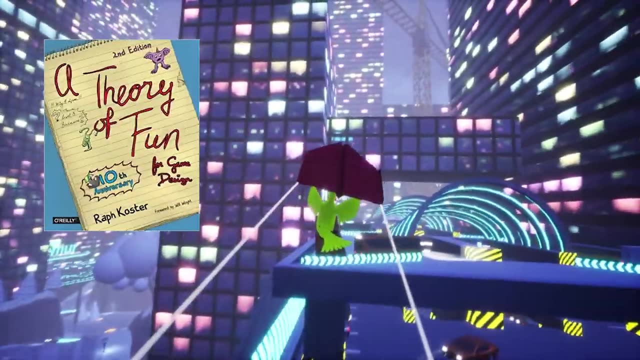 personal interests at a good pace without providing ways to cheat. As the creative director for the Star Wars Galaxies, Raph Costa, described in his famous book A Theory of Fun, all the possible patterns in games can be placed into one of six categories, which have all been helpful for people. 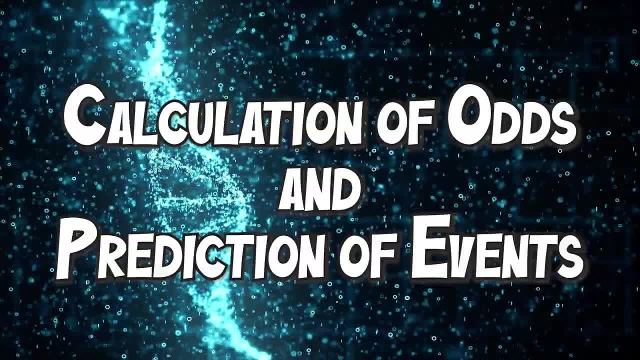 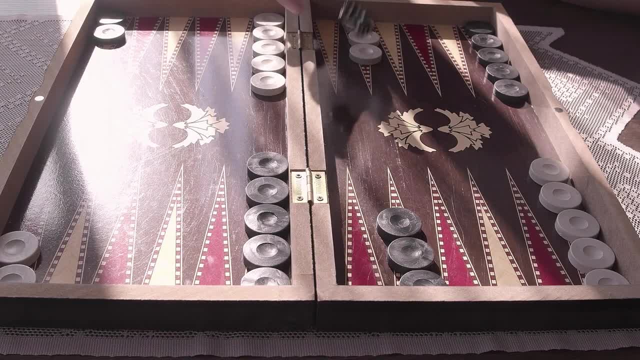 at some point throughout evolution. The first of these categories is the calculation of odds and prediction of events. This pattern applies to any game involving probability. A good example of this, where players need to roll a dice and then make a prediction of the best possible moves to win the 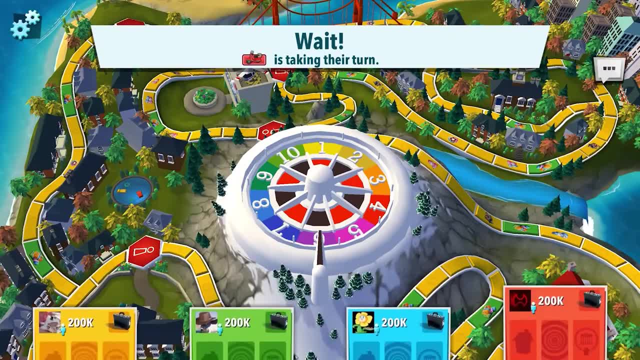 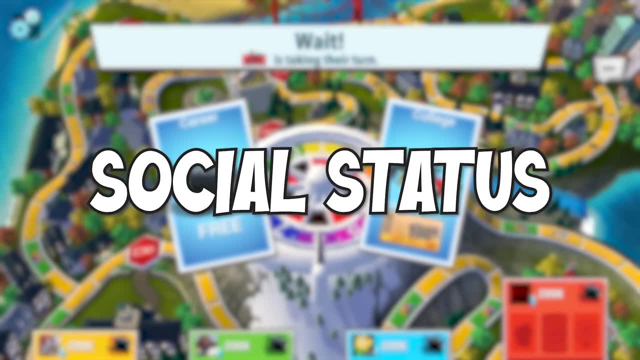 game. This category has many applications in real life where you need to weigh in the risks against the rewards, such as going to college or going straight to work. The second category is social status patterns, which have to do with pushing yourself and others up and down a ladder. 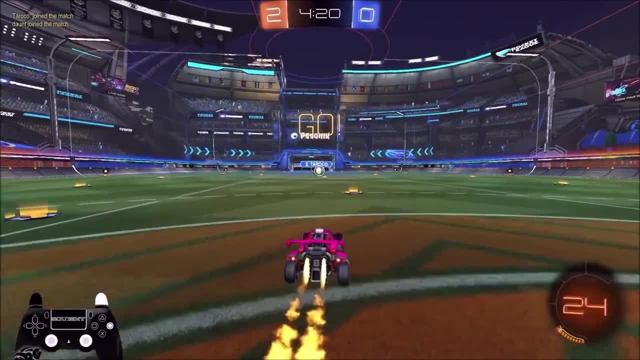 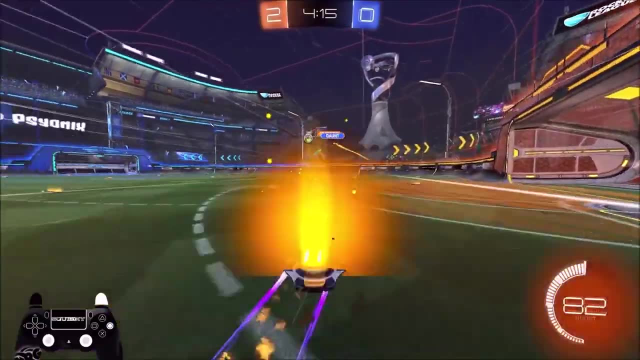 thus signaling your own value to others around you. This pattern involves a variety of positive and negative emotions and is arguably the most dangerous and addictive pattern in 21st century video games. A good example of this is the Overwatch competitive ladder, where people have people get joy by seeing others go down the ranks whilst elevating their own. 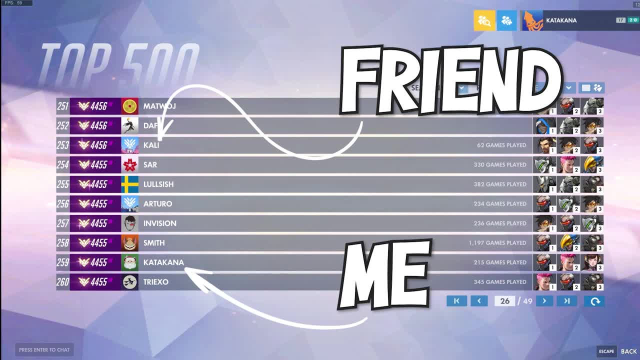 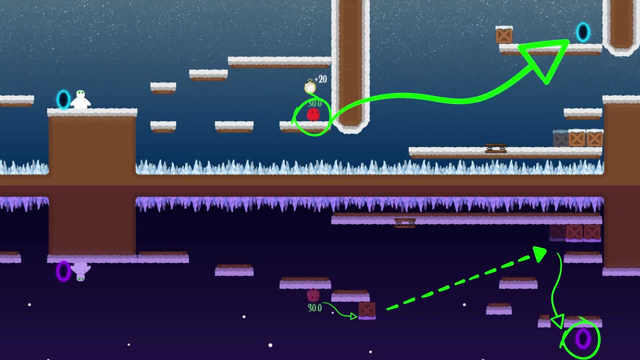 How many times has a friend made a joke at your expense, stating that their rank is higher than yours? The third category is spatial reasoning. These are patterns which require players to think ahead of time and determine possible results of an in game puzzle. This is done by analyzing what 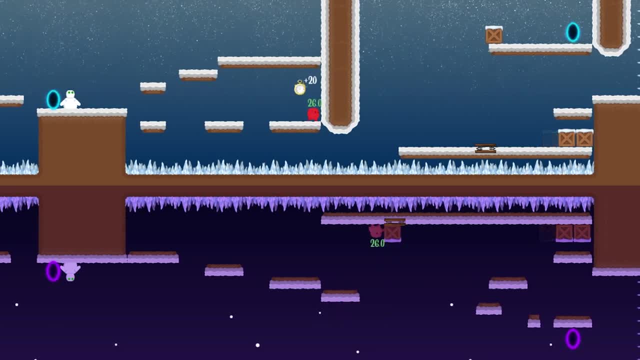 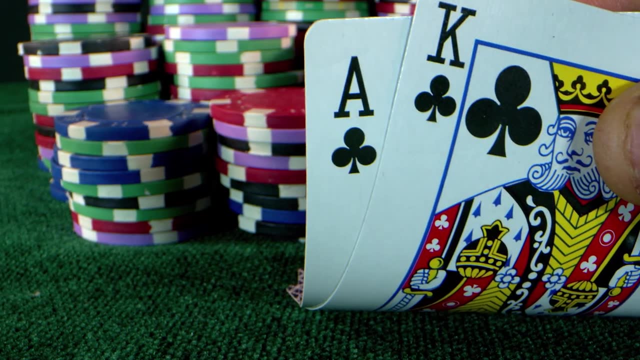 the possible moves are and figuring out what needs to be done to complete the puzzles. The fourth category is memory. These patterns involve recalling and managing complex chains of information, such as when counting cards in blackjack. This is rare in the video game, but is something that can be�� a new challenge. The fifth category is memory. These patterns involve 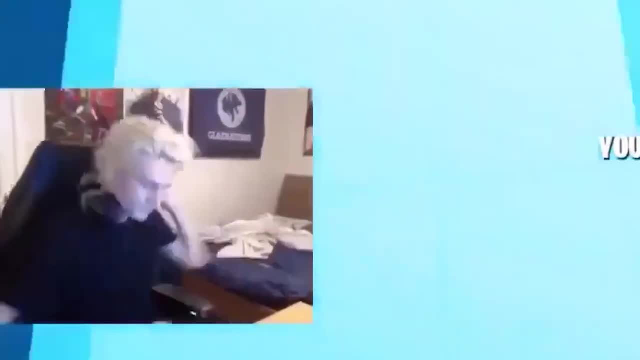 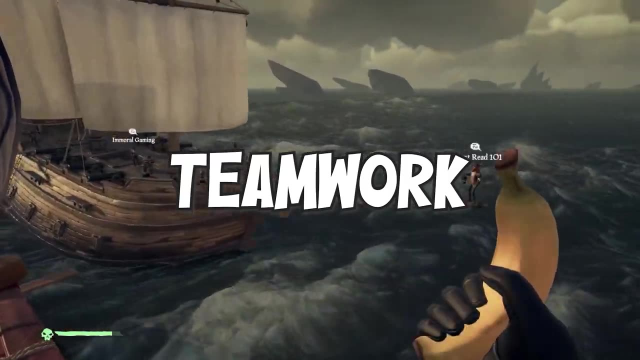 recalling and managing complex chains of information, such as when counting cards in blackjack. The fifth visceral responses, which occur when we have a physical reaction to a non-physical experience. shooter games fall under this category. and the final category is teamwork, which involves working with others to achieve a goal. this pattern is widely used in multiplayer games. these categories 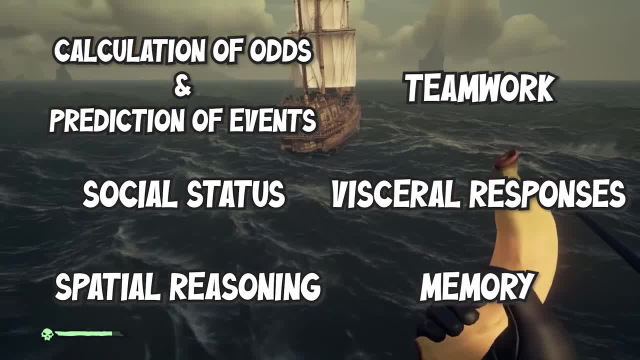 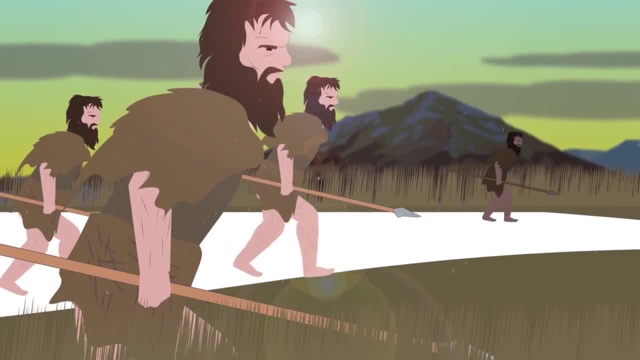 are universally helpful patterns to learn and have also been helpful in human evolution. consider how useful teamwork and memory were when humans were cavemen. if they hadn't utilized these, then they wouldn't have been able to hunt for food. in video games, these patterns are implemented through the 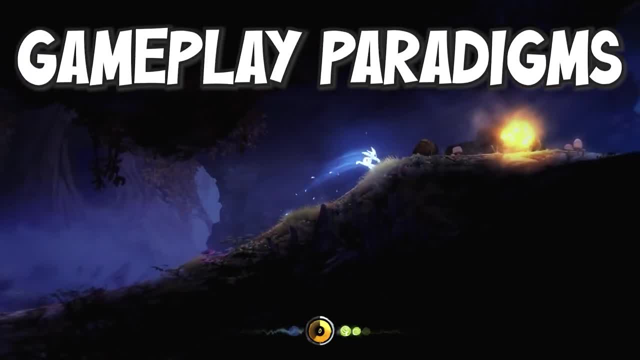 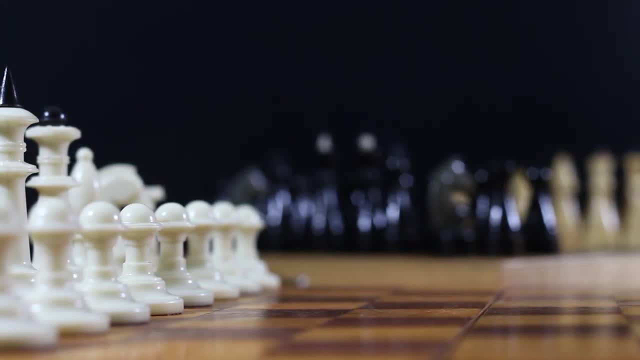 use of building blocks, known as game mechanics, in combination with gameplay paradigms. an example of a game mechanic is moving a piece on a chessboard, whereas game paradigms sometimes refer to as the core dynamics within a game, define the actual victory condition, such as taking your opponent's. 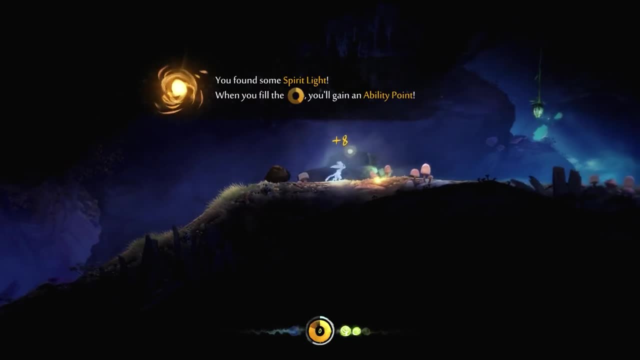 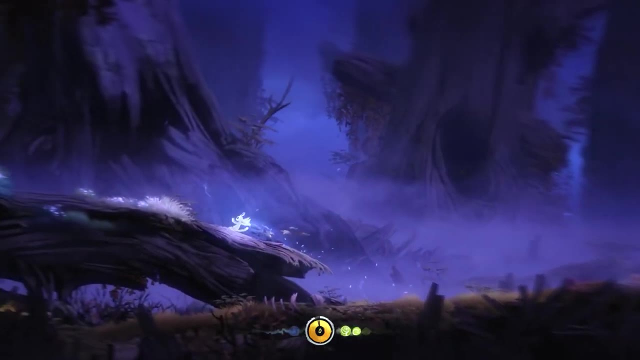 king in chess, the holy grail is a game that provides never-ending challenges, requires a wide range of skills to succeed and has a difficulty curve that perfectly adjusts to the player's skill level over time. this is why many great games with everlasting popularity are competitive head-to-head games. because of the high level of difficulty and the high level of 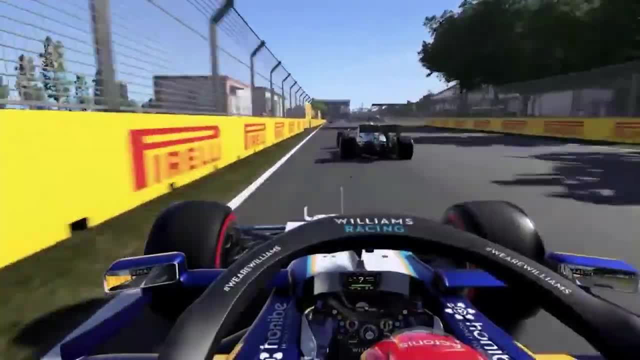 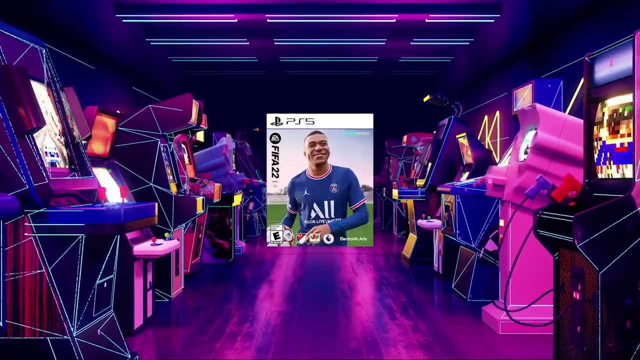 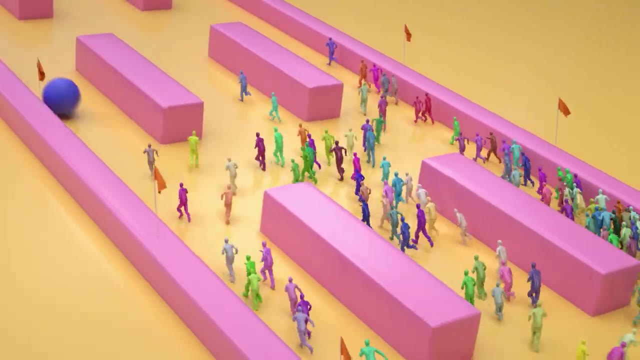 having other opponents provides an infinite number of challenges with a continuous range of difficulties. however, this doesn't mean that every head-to-head game will thrive. despite the vast number of games, new games typically only slightly improve upon previous competitors. this is due to game designers commonly being culprits of unoriginality. they play more games than the 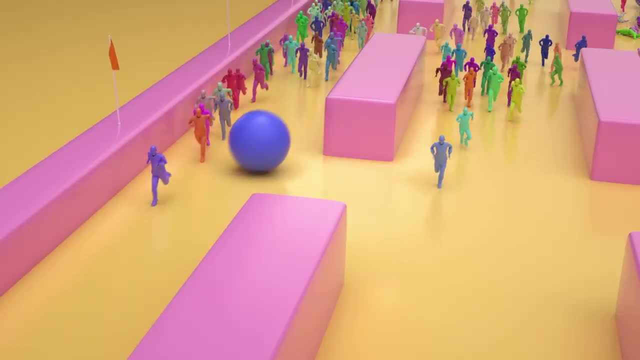 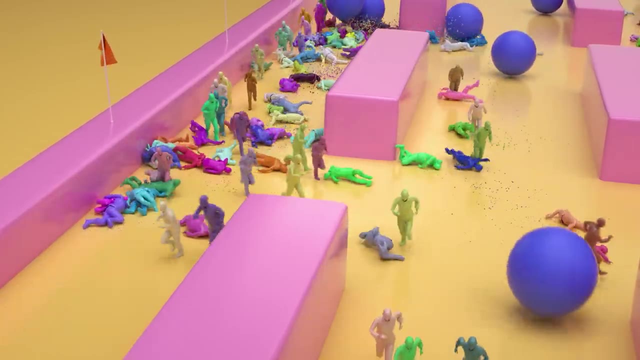 average player sample mechanics from those games, then use them to build their games. when this happens, games don't introduce new ideas and thus wither away, as people have previously learned the mechanics which the game teaches, and so they get bored. in order to make games fun, designers need to find new dimensions to add to the gameplay. 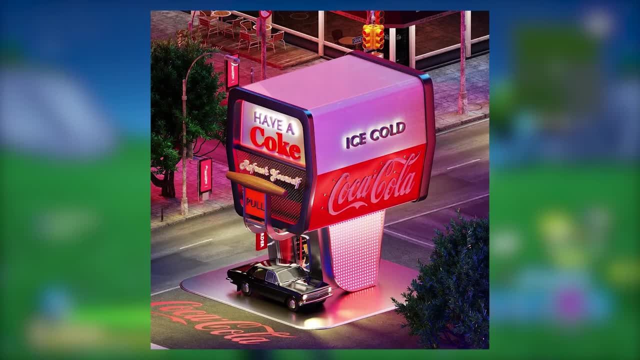 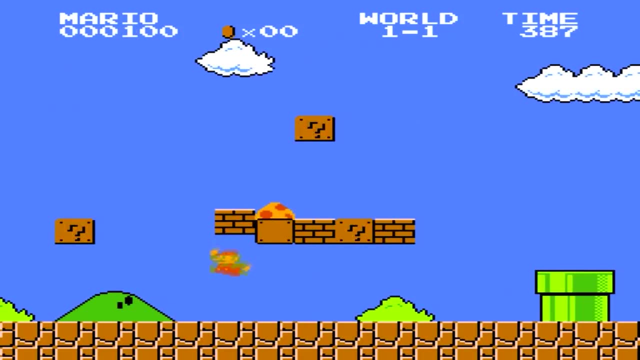 this isn't achieved by adding more weapons to a battle royale, but rather by coming up with innovative ways to combine different mechanics. take super mario, for example: changing the blocks into hexagons isn't a big change and is not likely to teach the players new things. however, take that. 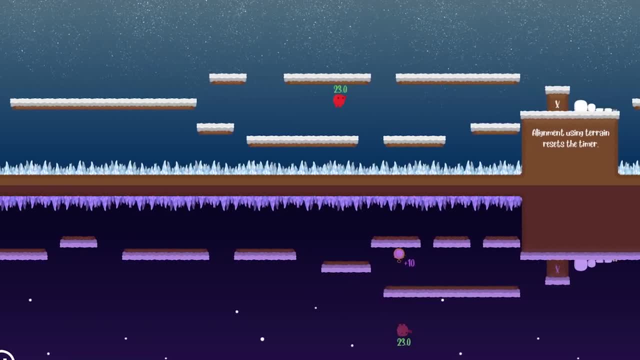 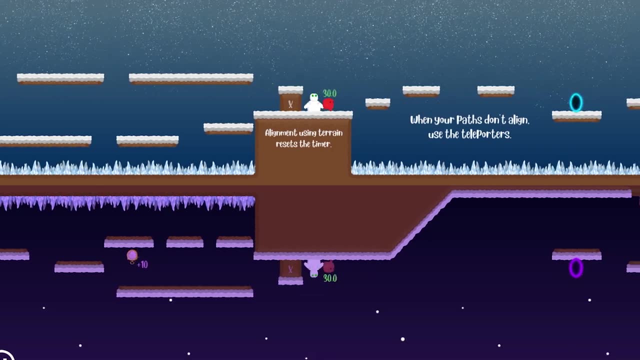 same game and add a new dimension to it, such as having to control the character in two separate worlds simultaneously, and the pattern changes completely. however, even with innovation, it's impossible for any game to afford a new dimension to the game as a whole. however, even with innovation, it's impossible for any game to